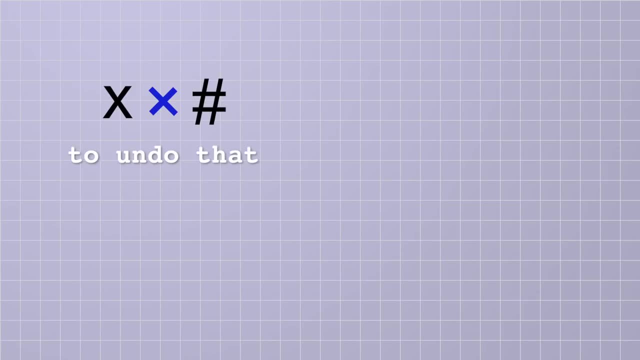 If an unknown is being multiplied by a number, to undo that, we need to divide both sides by that number. But if an unknown is being divided by a number, to undo that, we need to multiply both sides by that number. Now don't worry if that sounds a little confusing right now. 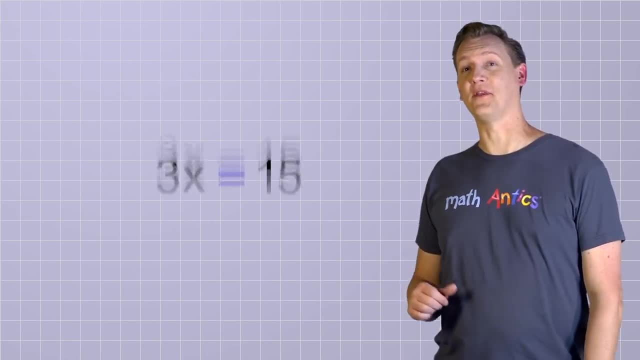 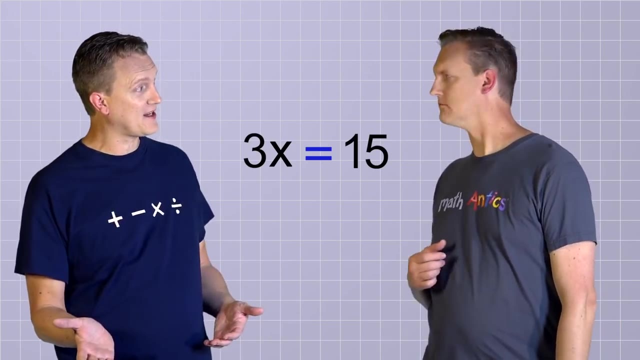 It'll make a lot more sense after you've seen a few examples. Let's start with this one: 3x equals 15.. Uh, excuse me, I think you forgot something. I mean, didn't you say that these equations were going to have multiplication or division in them? 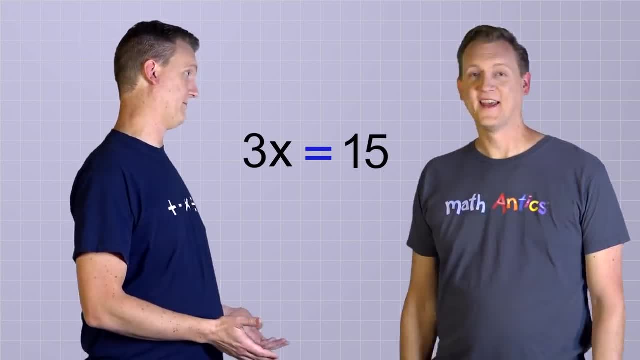 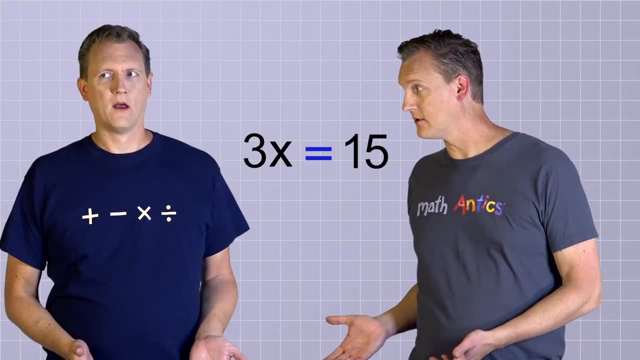 But I don't see any arithmetic operator at all in this equation. Actually, I think you forgot something that we learned in the video What Is Algebra? You did watch that, right? Oh, sure, sure, of course, But I… you know, I just remembered. 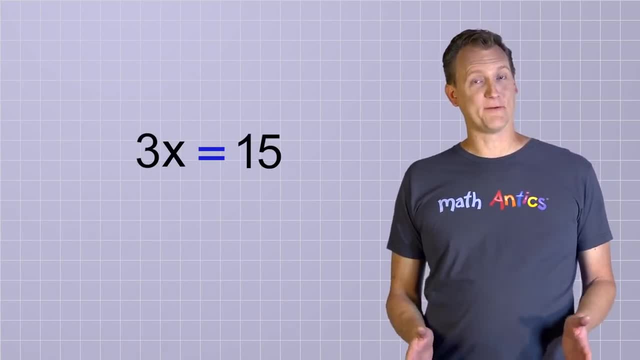 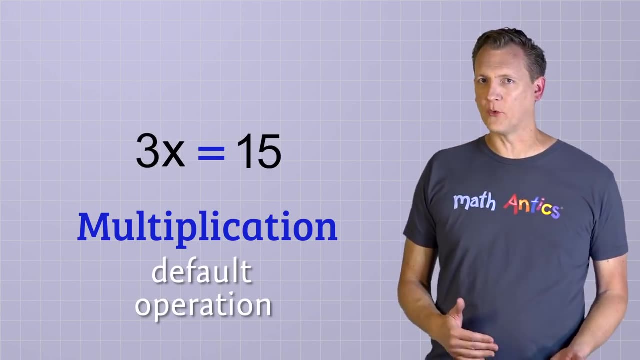 I have something I gotta do. I'll be right back. Well, I'm sure you remember that multiplication is the default operation in algebra. See a number and a symbol right next to each other like this, With no operation between them. it means they're being multiplied. 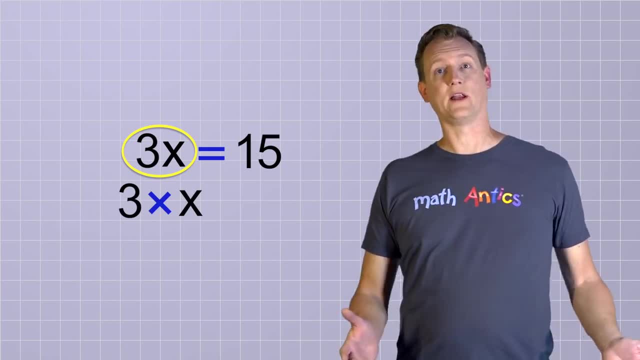 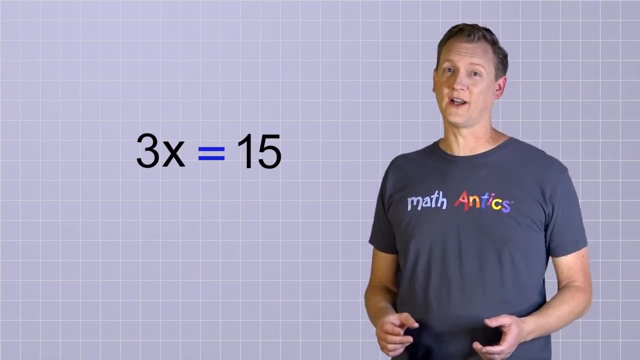 So 3x is the same as 3 times x. Oh, and just a side note: Since in multiplication the order of the numbers doesn't matter, you COULD switch the order and write x3,, but it's customary to always list the known number first, and 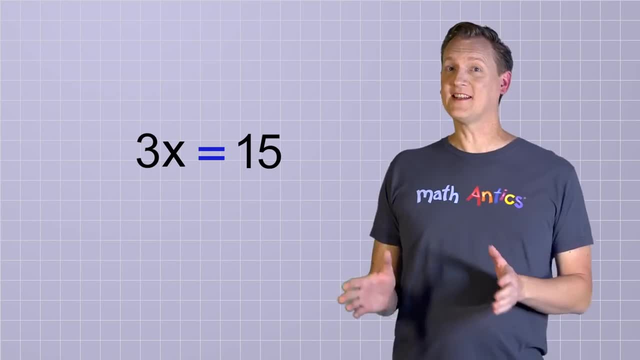 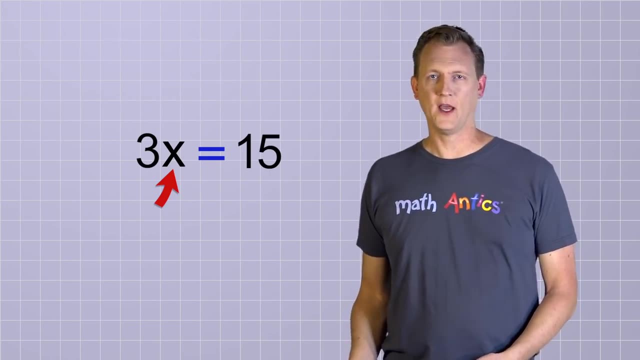 the unknown number second. Alright, but we need to solve this equation right. That means we need to get the unknown x all by itself on one side of the equal sign. Right now the x is NOT by itself because it's being multiplied by 3.. 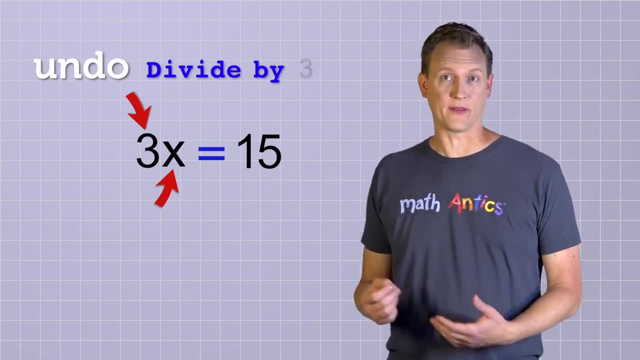 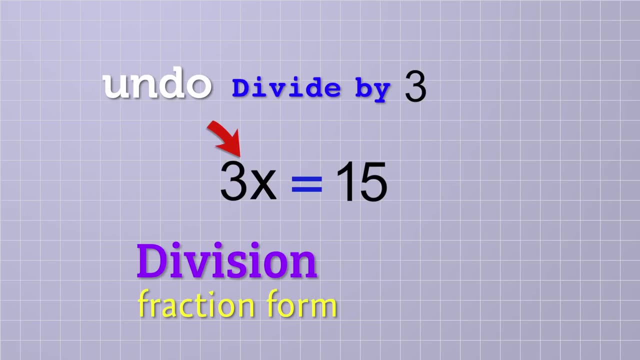 So to undo that operation we need to divide that side by 3.. In algebra we almost always write division in fraction form. So to divide this side by 3, we just write a fraction line under it and we put a 3 below. 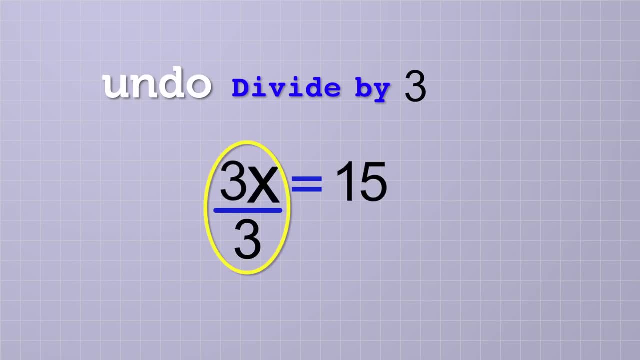 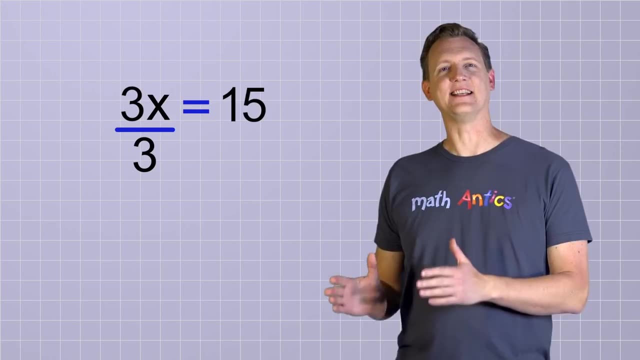 the line There. This means 3 times x divided by 3.. Ah, but don't forget our rule for rearranging equations: We have to do the exact same thing to the other side to keep the equation balanced. That's better. 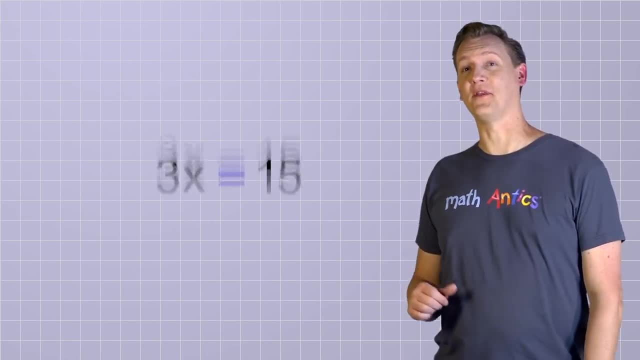 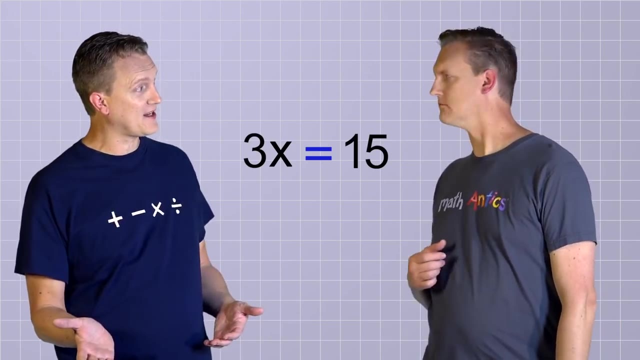 It'll make a lot more sense after you've seen a few examples. Let's start with this one: 3x equals 15.. Uh, excuse me, I think you forgot something. I mean, didn't you say that these equations were going to have multiplication or division in them? 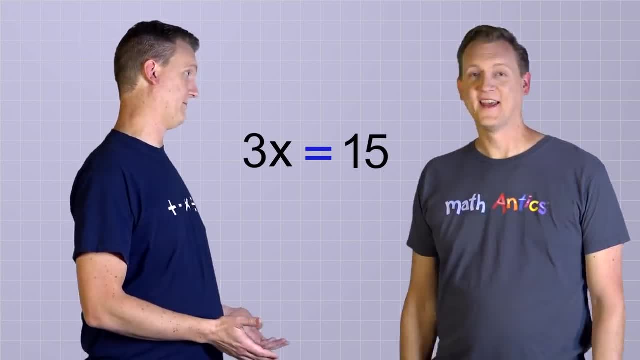 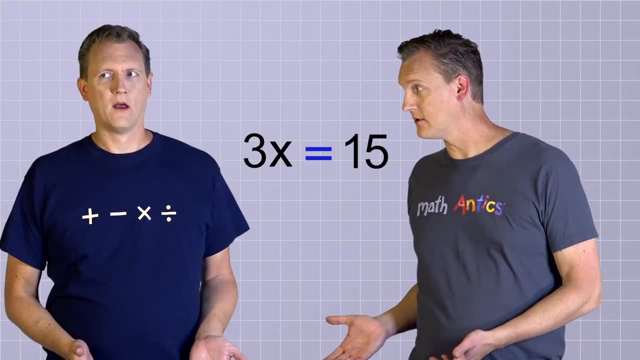 But I don't see any arithmetic operator at all in this equation. Actually, I think you forgot something that we learned in the video What Is Algebra? You did watch that, right? Oh, sure, sure, of course, But I… you know, I just remembered. 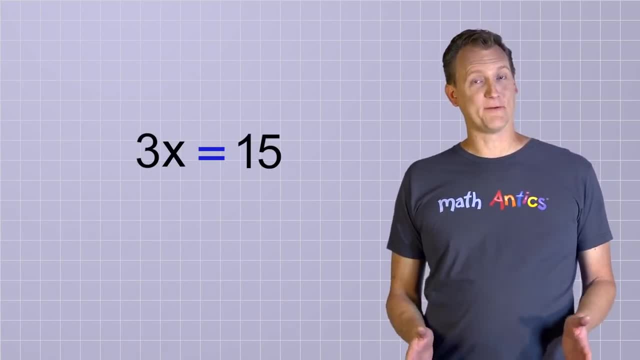 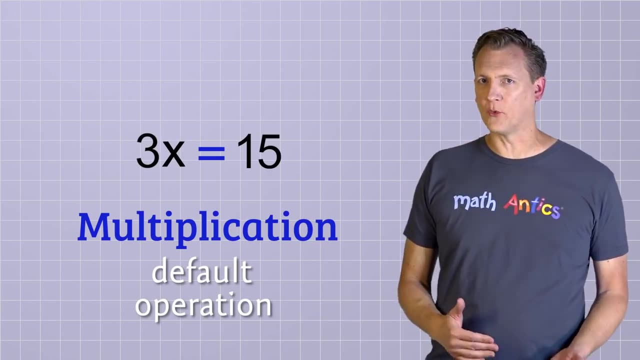 I have something I gotta do. I'll be right back. Well, I'm sure you remember that multiplication is the default operation in algebra. See a number and a symbol right next to each other like this, With no operation between them. it means they're being multiplied. 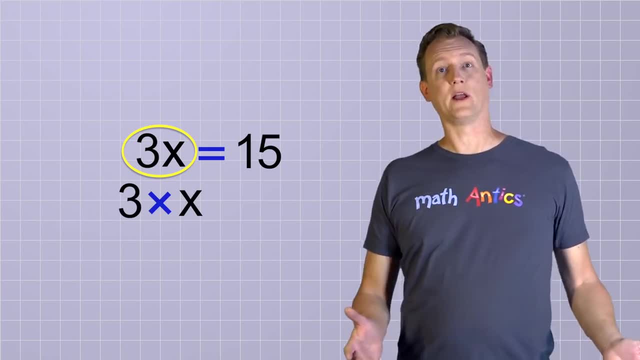 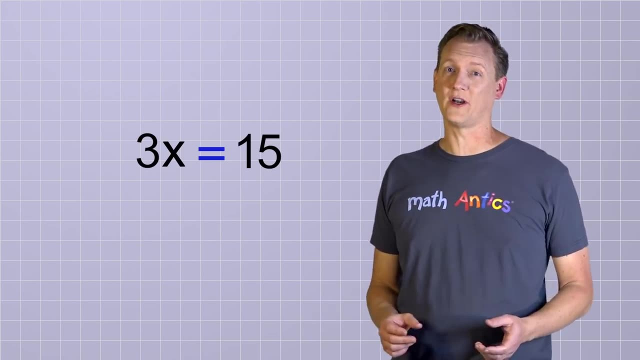 So 3x is the same as 3 times x. Oh, and just a side note: Since in multiplication the order of the numbers doesn't matter, you COULD switch the order and write x3,, but it's customary to always list the known number first, and 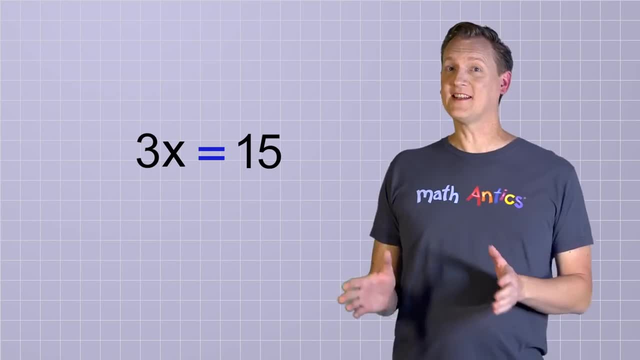 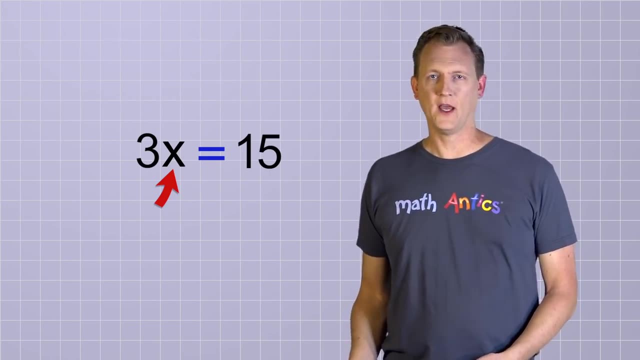 the unknown number second. Alright, but we need to solve this equation right. That means… We put the unknown x, all by itself, on one side of the equal sign. Right now, the x is NOT by itself because it's being multiplied by 3.. 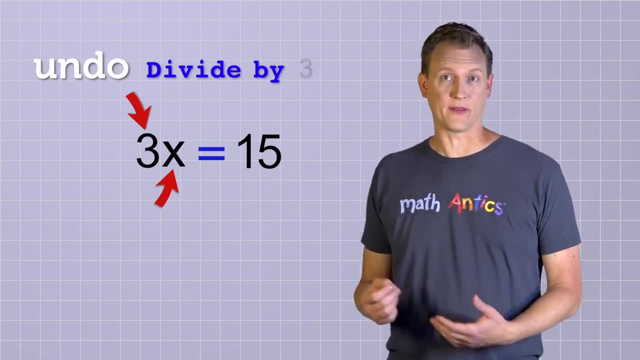 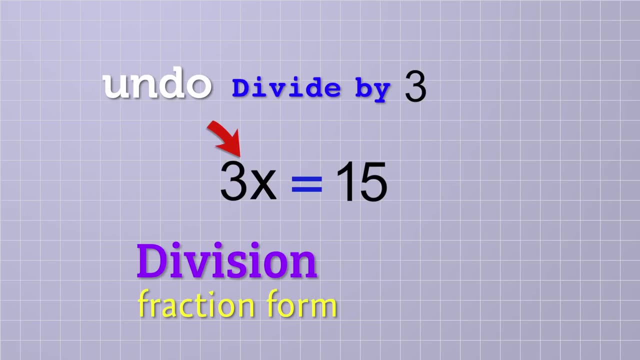 So to undo that operation we need to divide that side by 3.. In algebra we almost always write division in fraction form. So to divide this side by 3, we just write a fraction line under it and we put a 3 below. 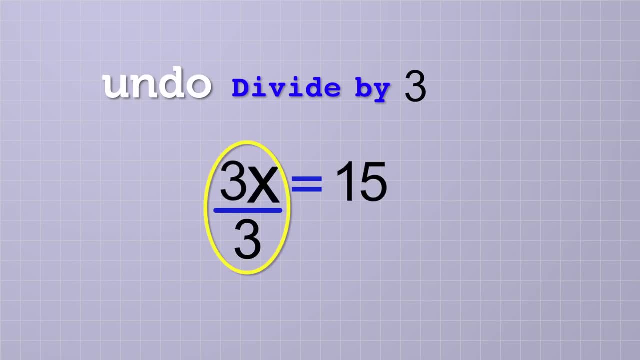 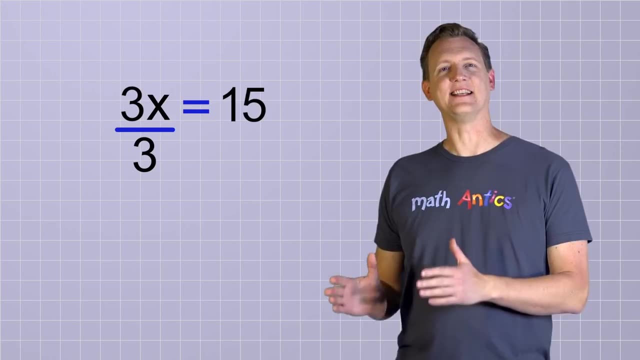 the line There. This means 3 times x divided by 3.. Ok, Ah, but don't forget our rule for rearranging equations: We have to do the exact same thing to the other side to keep the equation balanced. That's better. 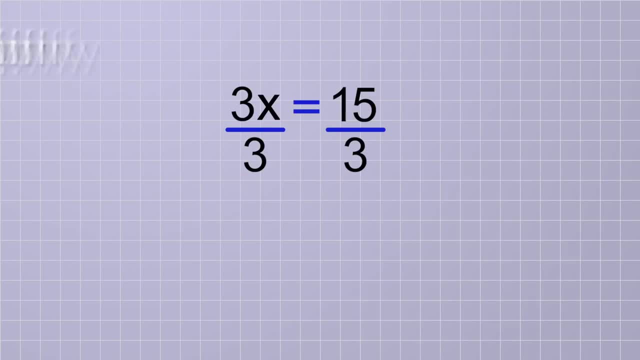 Now both sides are being divided by 3.. The next step is to simplify: The 3 on the top and the 3 on the bottom on this side cancel, because 3 divided by 3 would just be 1.. This is just like cancelling common factors when you're simplifying a fraction. 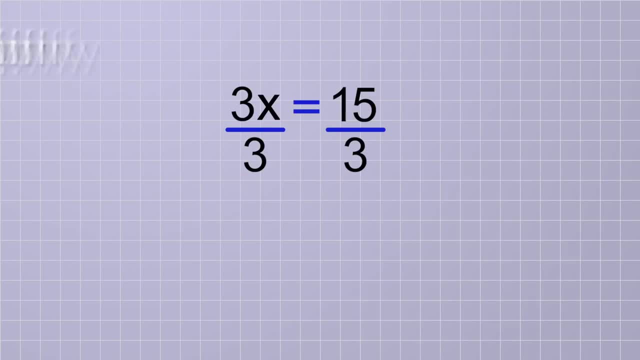 Now both sides are being divided by 3.. The next step is to simplify: The 3 on the top and the 3 on the bottom on this side cancel, because 3 divided by 3 would just be 1.. This is just like cancelling common factors when you're simplifying a fraction. 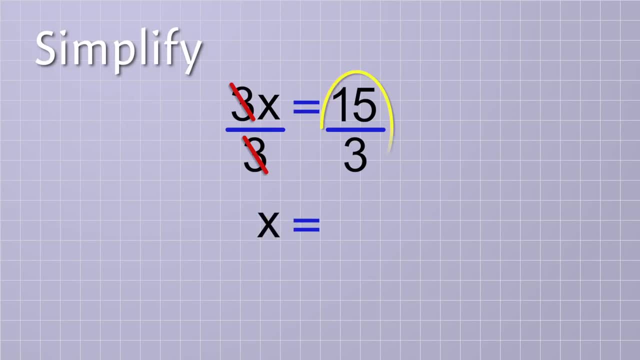 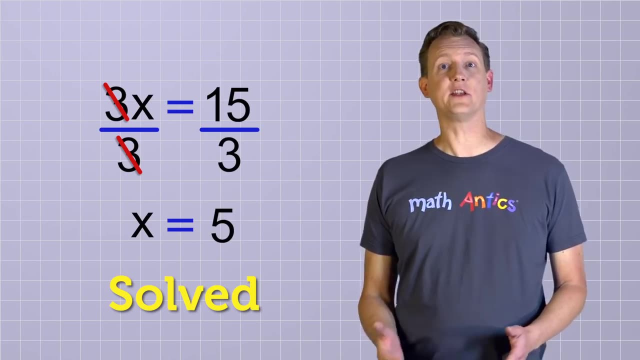 That leaves us with just x on this side, And on the other side we have 15 divided by 3, which simplifies to 5.. There We've solved our equation by changing it into the simplified form: x equals 5.. 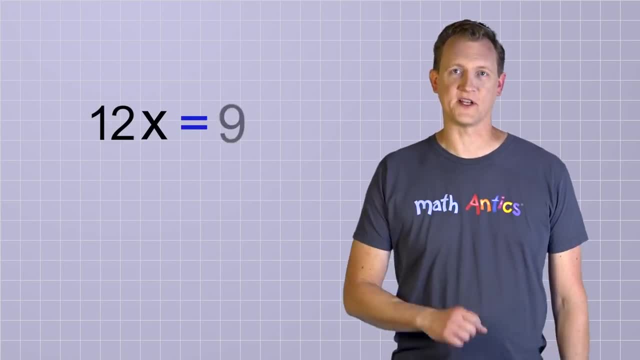 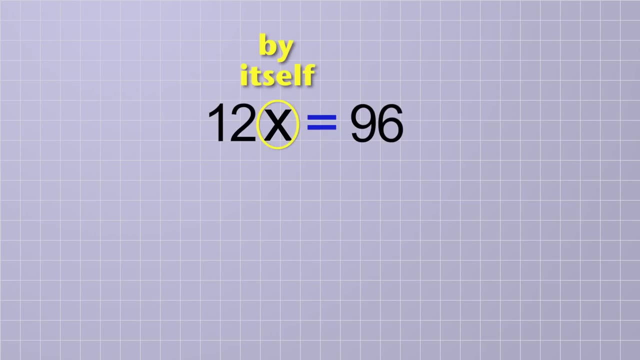 Let's try another one, just like that. 12x equals 96.. In this problem, the unknown is being multiplied by 12. So to get the x all by itself, we're going to need to divide both sides of the equation by 12.. 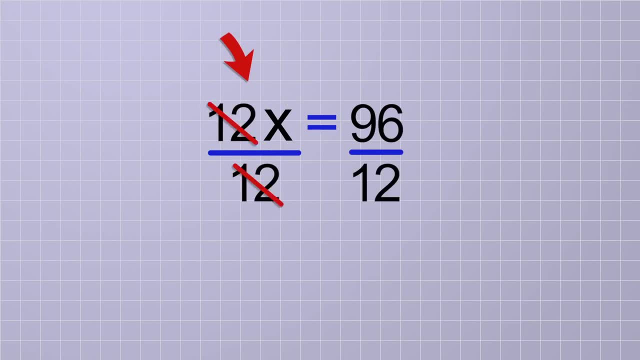 On the first side, the 12 on top and the 12 on bottom cancel out, leaving just x. That's good, And on the other side, we need to divide 96 by 12.. You might be able to do that by memory, but if not, you can use a calculator to divide. 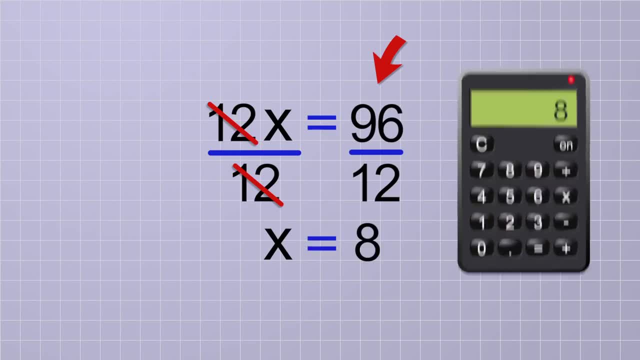 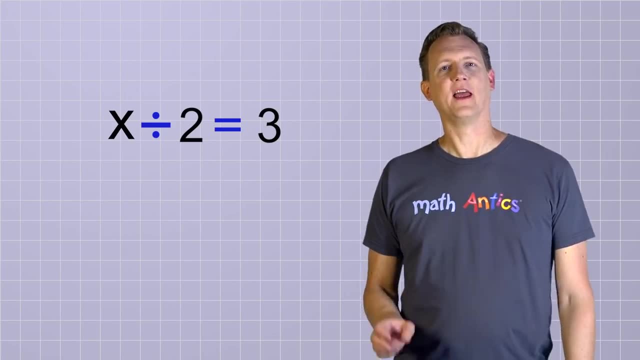 96 divided by 12 is 8.. So in this problem x equals 8.. That's pretty easy, isn't it? Are you ready to try a division problem now? Here we have: x divided by 2 equals 3.. 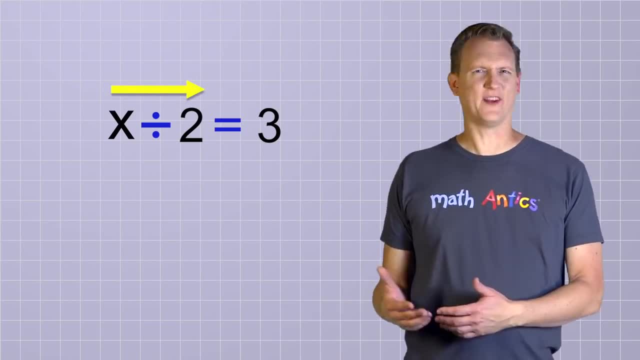 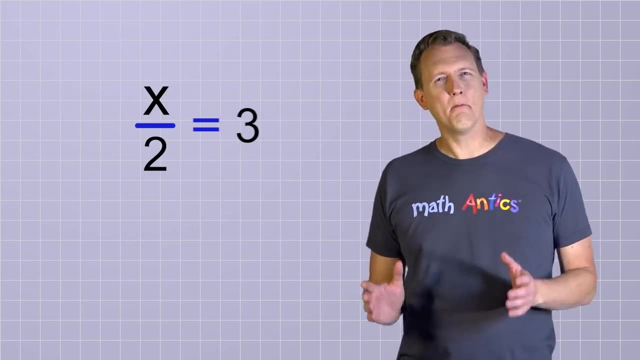 Now, when you see division written like this from left to right with the traditional division symbol, I want you to rewrite it using the fraction form for division, And that's because it's much easier to cancel common factors and simplify your equation when you use the fraction form. 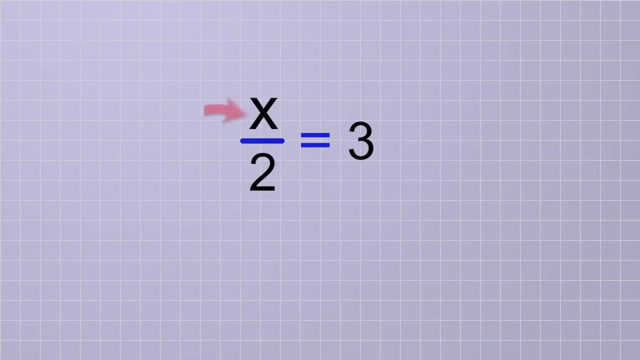 Now that we have it rewritten, let's solve it. We can see that the unknown is not by itself, because it's being divided by 2. How can we get rid of or undo that division? Yep, we can undo division with multiplication. 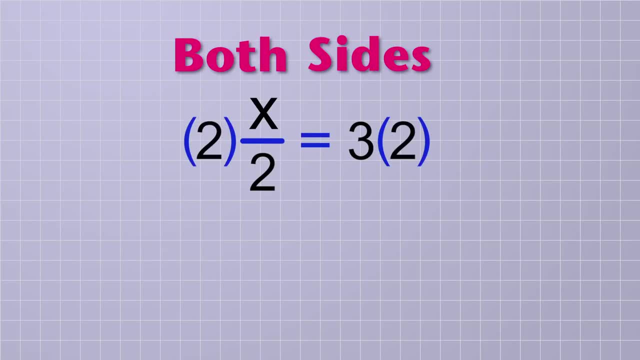 So we need to multiply both sides of the equation by 2.. Instead of writing the multiplication sign, I'm using the parenthesis notation that we learned about in the video called What is Algebra? Remember the multiplication is just implied. Now, to simplify. 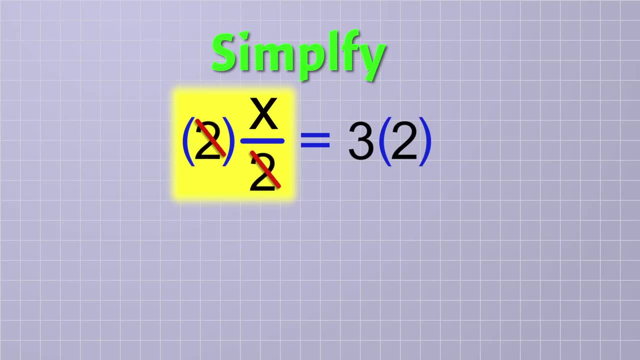 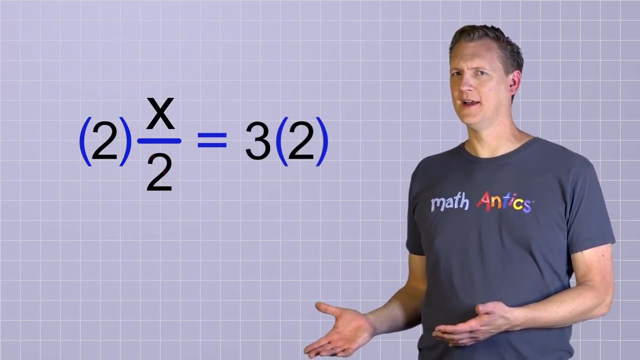 On the first side. the 2 on top cancels out the 2 on the bottom, since 2 divided by 2 is just 1.. And I know what some of you are thinking: How is there a 2 on top? 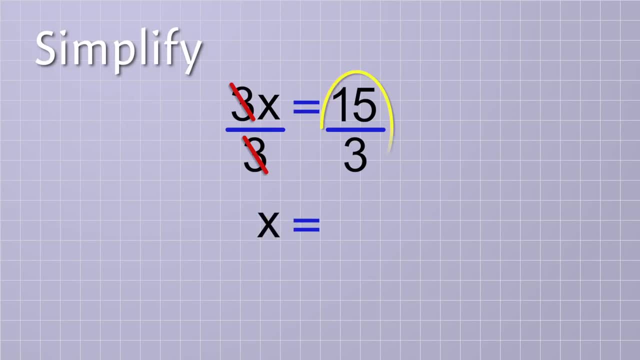 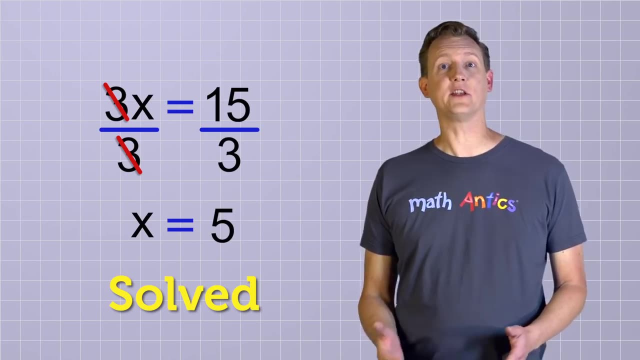 That leaves us with just x on this side, And on the other side we have x on this side. Ok, So on this side we have 15 divided by 3, which simplifies to 5.. There We've solved our equation by changing it into the simplified form: x equals 5.. 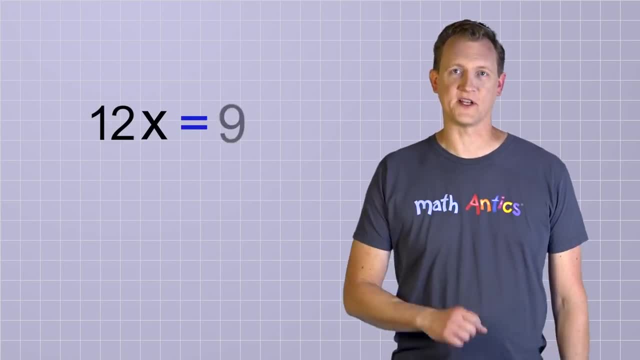 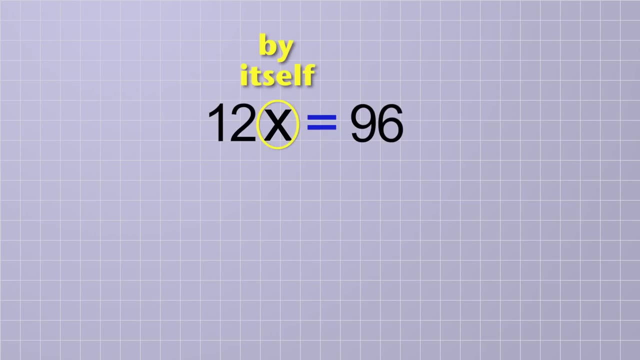 Let's try another one, just like that. 12x equals 96.. In this problem, the unknown is being multiplied by 12. So to get the x all by itself, we're going to need to divide both sides of the equation by 12.. 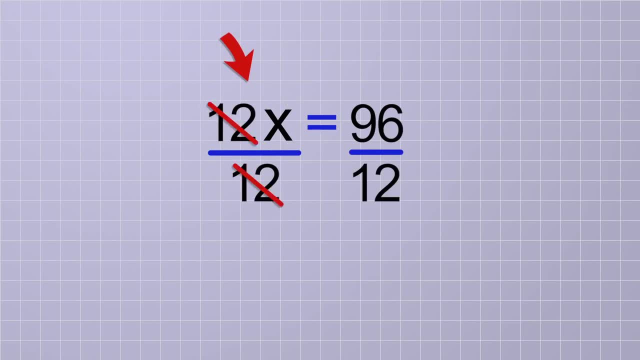 On the first side, the 12 on top and the 12 on bottom cancel out, leaving just x on that side, And on the other side we need to divide 96 by 12.. You might be able to do that by memory, but if not, you can use a calculator to divide. 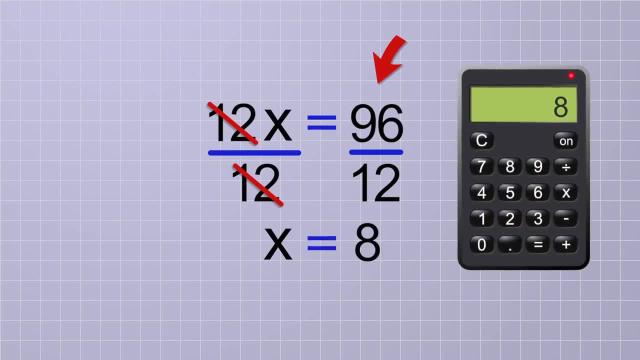 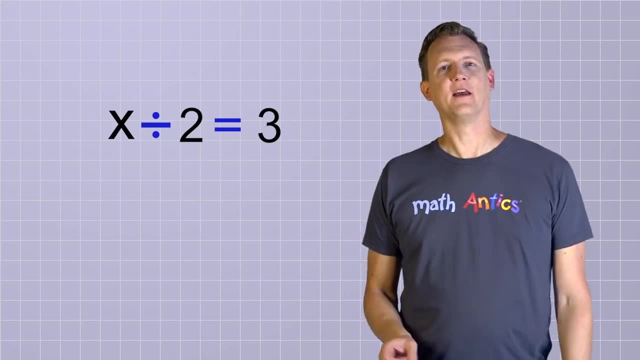 96 divided by 12 is 8.. So in this problem x equals 8.. That's pretty easy, isn't it? Are you ready to try a division problem now? Here we have: x divided by 2 equals 3.. 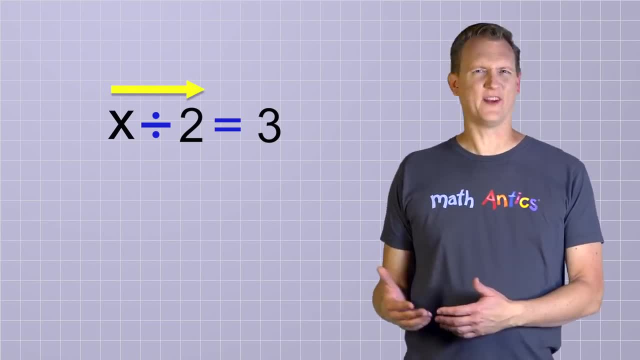 Now, when you see division written like this, from left to right, with the traditional division symbol, I want you to rewrite it using the same formula. I want you to rewrite it using the same formula. I want you to rewrite it using the fraction form for division. 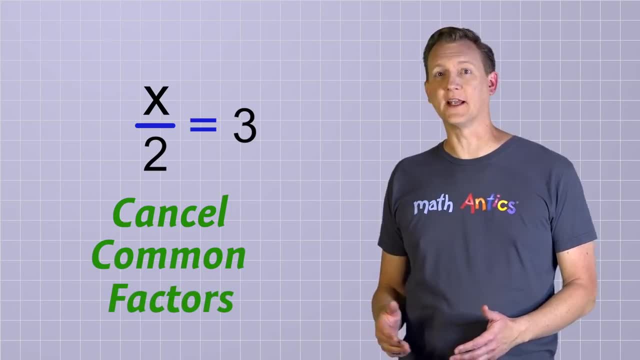 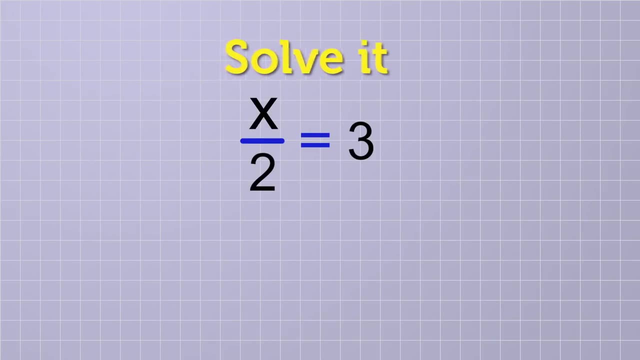 And that's because it's much easier to cancel common factors and simplify your equation when you use the fraction form. Now that we have it rewritten, let's solve it. We can see that the unknown is not by itself, because it's being divided by 2.. 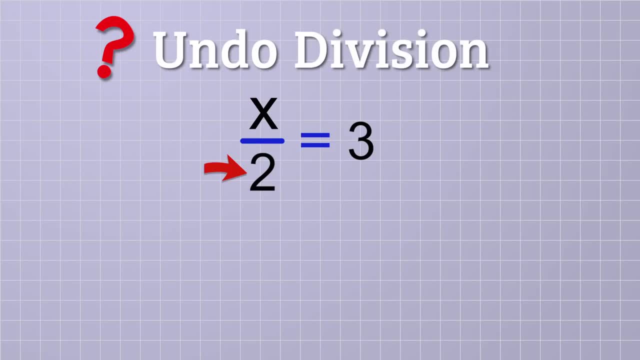 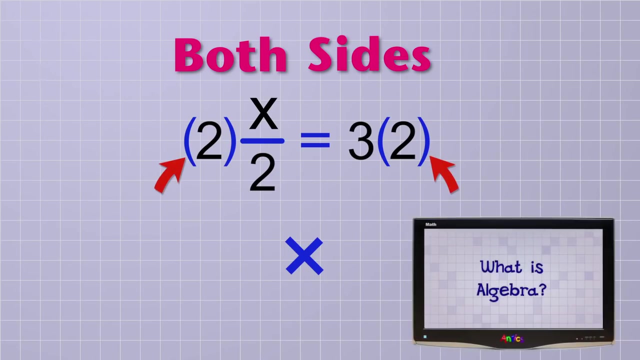 How can we get rid of or undo that division? Yup, we can undo division with multiplication. So we need to multiply both sides of the equation by 2.. Instead of writing the multiplication sign, I'm using the parentheses notation that we learned about in the video called What is Algebra? 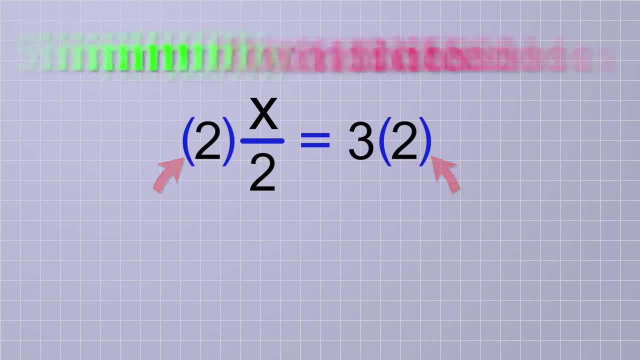 Remember the multiplication is just implied. Now, to simplify, On the first side, the 2 on top cancels out the 2 on the bottom, since 2 divided by 2 is just 1.. And I know what some of you are thinking. 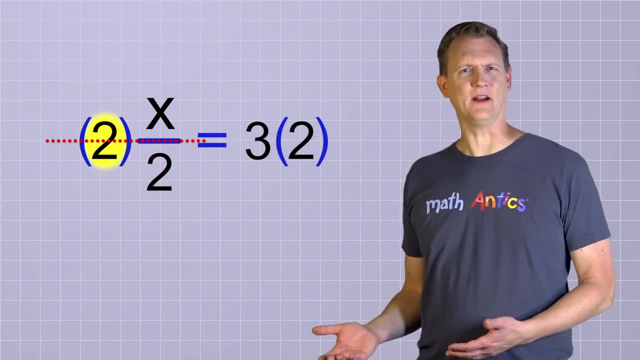 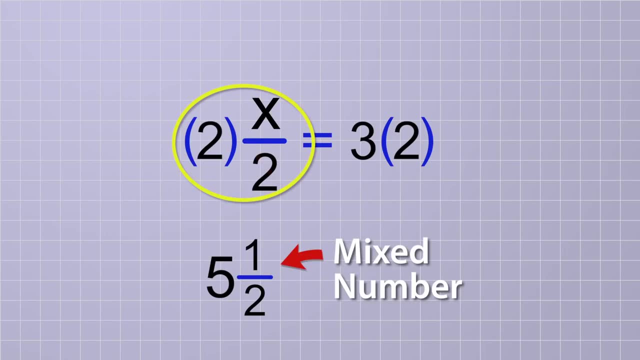 How is there a 2 on top? The 2 looks like it's really in the middle, Kind of like how a mixed number looks. That's true, But don't confuse this with a mixed number. Mixed numbers involve addition, but the parentheses let you know that the 2 and the x over 2 are being multiplied, since multiplication is the default operation. 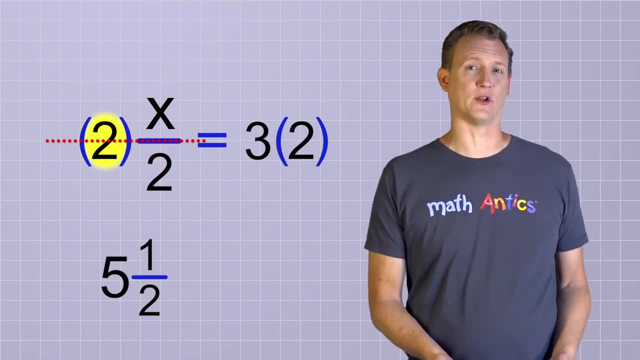 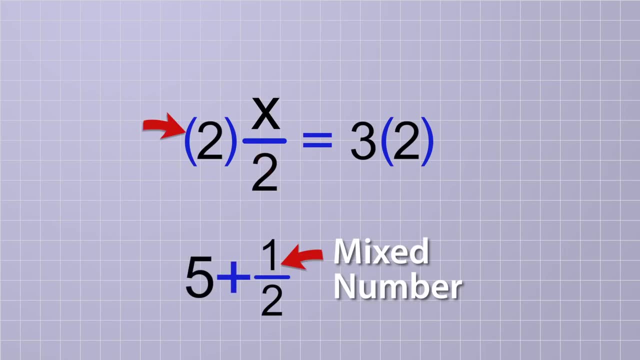 The 2 looks like it's really in the middle… kind of like how a mixed number looks. That's true, But don't confuse this with a mixed number. Mixed numbers involve addition, but the parenthesis let you know that the 2 and the x over 2 are. 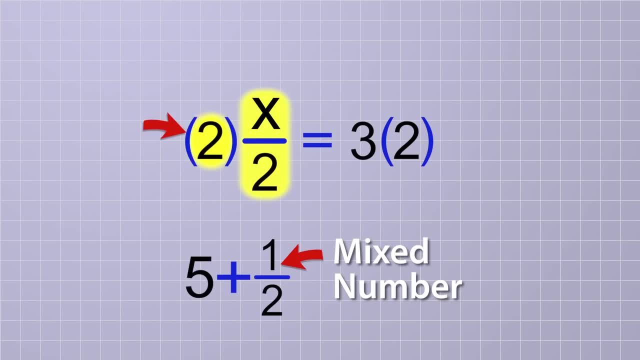 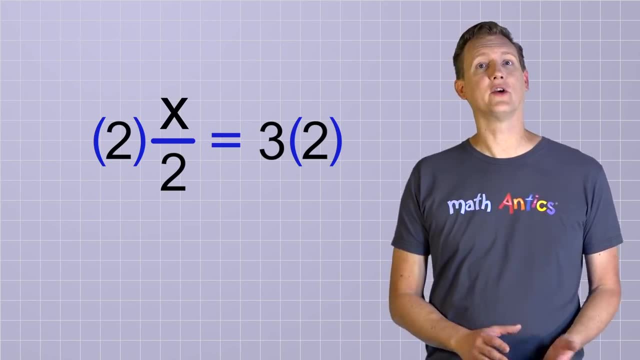 being multiplied, since multiplication is the default operation. OK, so it's not a mixed number, but how is the 2 on top? Well, do you remember how you can turn any number into a fraction? just by making 1 the bottom number. 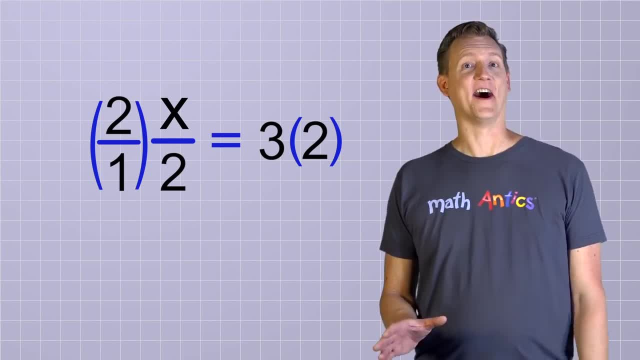 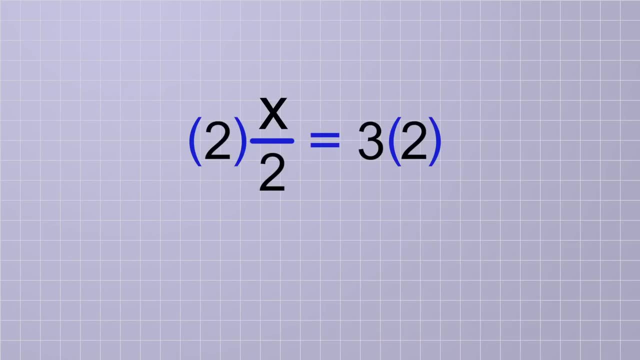 That means that 2 is the same as 2 over 1.. Ah, now you can see that the 2 really is on top. It's just that we don't usually show the 1 on the bottom. Alright, then, so the 2's cancel, leaving the x all by itself on this side. 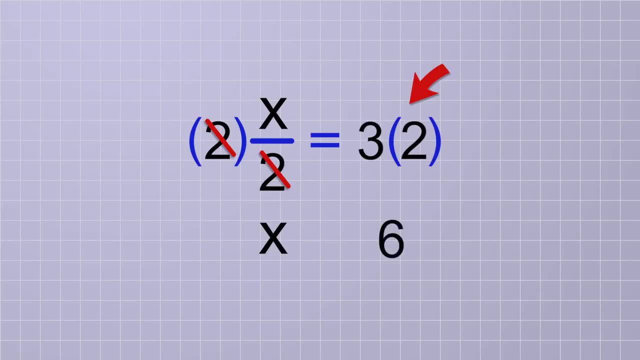 And on the other side we have 3 times 2,, which is just 6.. So in this problem x equals 6.. That's not too hard either. Let's try another one: x over 10 equals 15.. 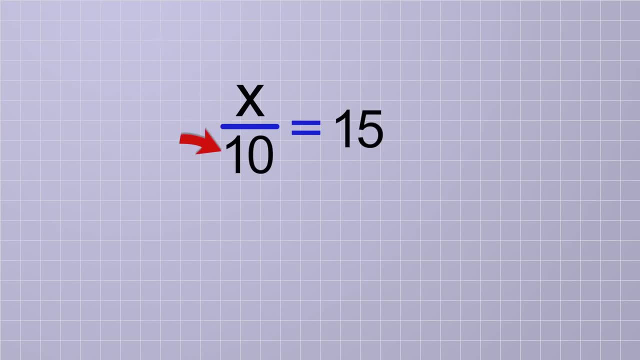 In this problem, since the x is being divided by 10, to get it by itself we're going to need to multiply both sides of the equation by 10.. On the first side, the 10's cancel, leaving x all by itself. 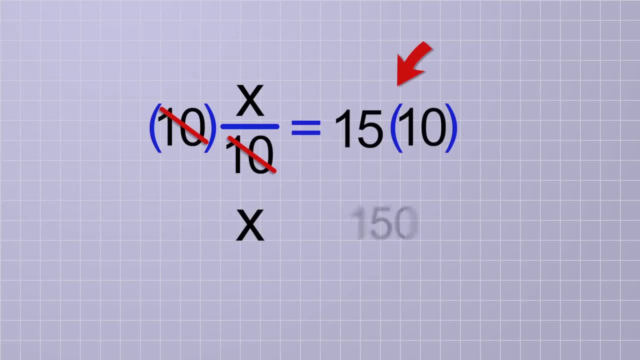 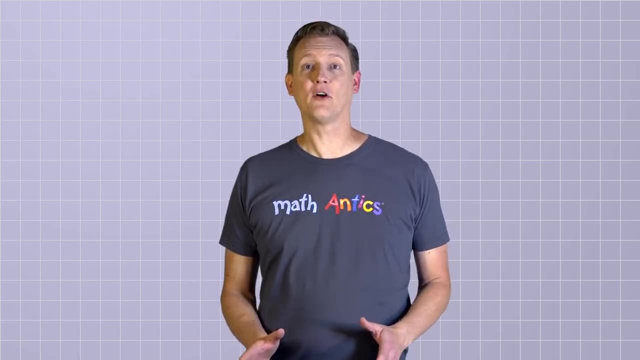 And on the other side we have 15 times 10, which is 150.. So our answer is: x equals 150.. Great, That's how you solve simple equations where an unknown is being multiplied by a number or divided by a number. 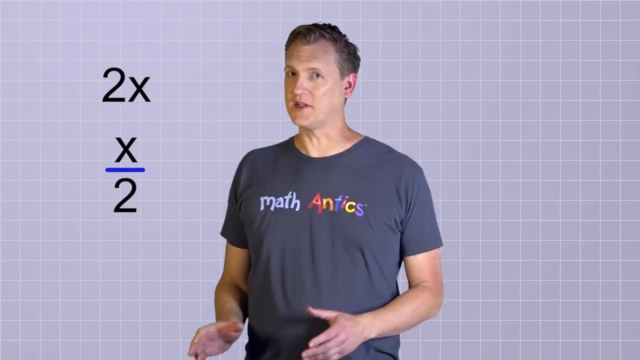 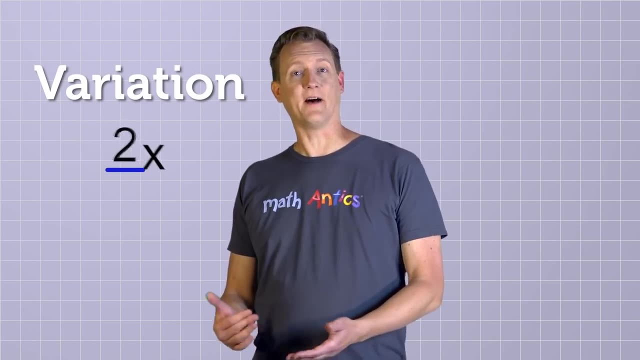 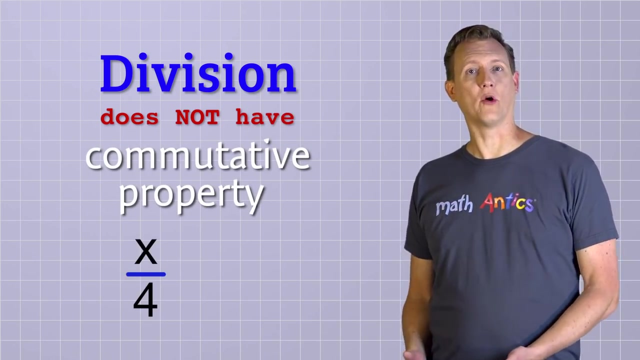 But just like with subtraction in the last video, with division there's a tricky variation that I need to tell you about. It's an equation where a number is being divided by an unknown, Since division does not have the commutative property. x over 4 is NOT the same thing as 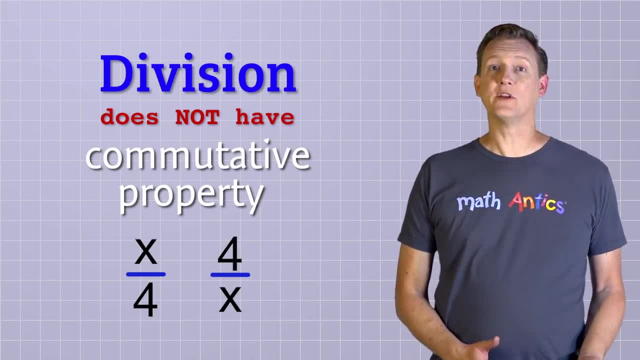 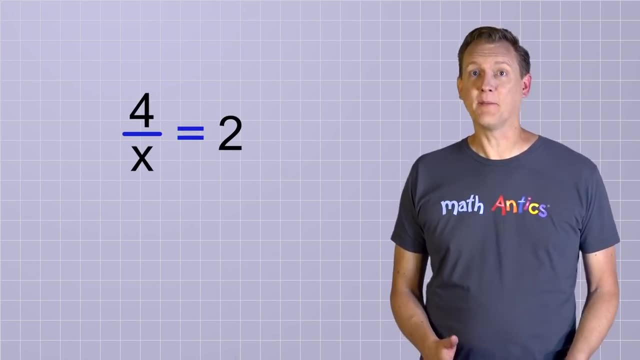 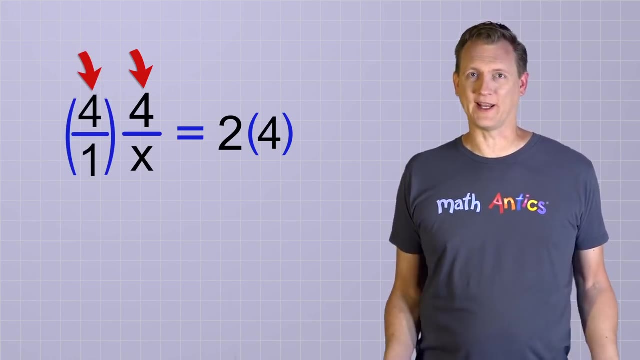 4 over x. So what do we do if the unknown is on the bottom, like in this problem? 4 over x equals 2.. Well, your first thought might be to multiply both sides by 4.. But that won't help us here, because both of the 4's would be on top, so they wouldn't. 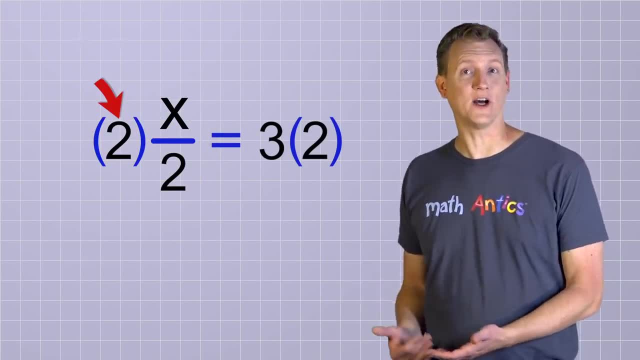 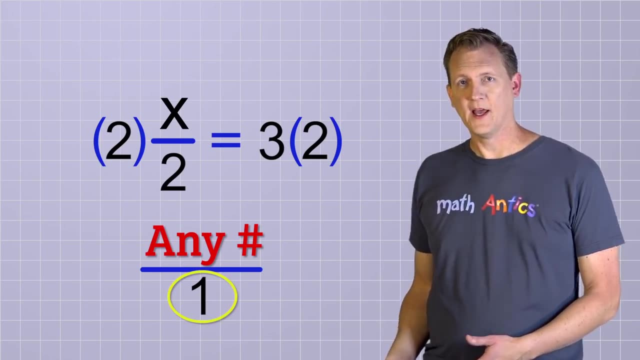 OK, so it's not a mixed number, but how is the 2 on top? Well, do you remember how you can turn any number into a fraction? just by making 1 the bottom number. That means that 2 is the same as 2 over 1.. 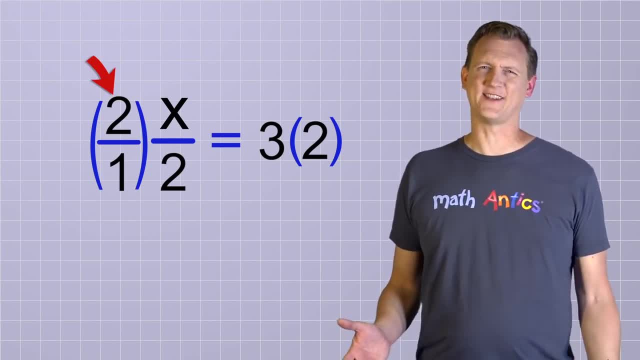 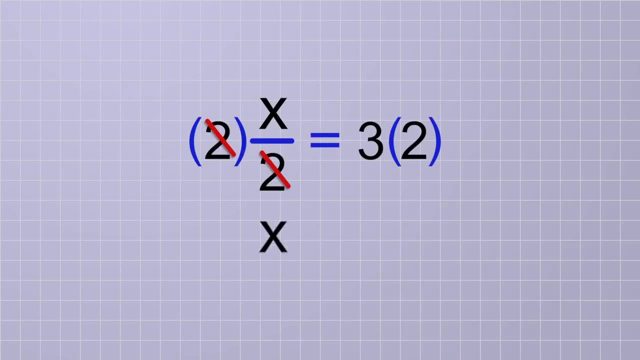 Ah, now you can see that the 2 really is on top. It's just that we don't usually show it. We show the 1 on the bottom. Alright, then, so the 2's cancel, leaving the x all by itself on this side. 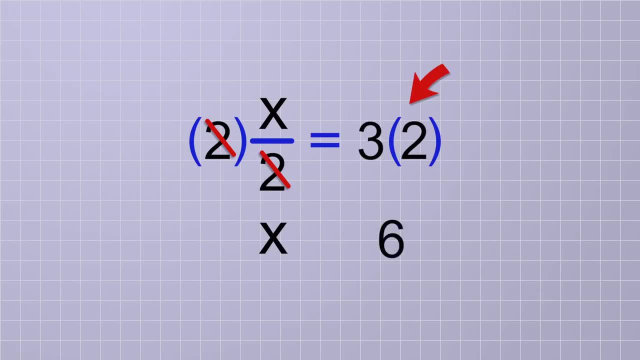 And on the other side we have 3 times 2,, which is just 6.. So in this problem x equals 6.. That's not too hard either. Let's try another one: x over 10 equals 15.. 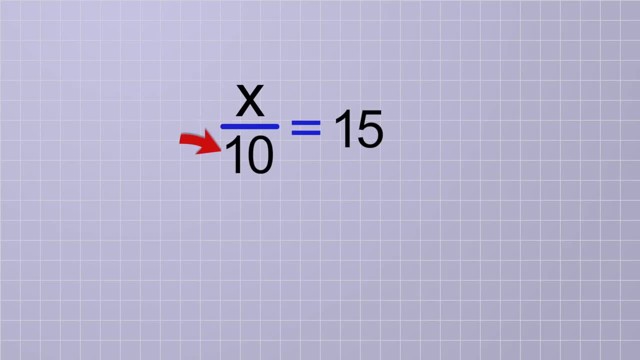 In this problem, since the x is being divided by 10, to get it by itself, we're going to need to multiply both sides of the equation by 10.. The 10's cancel, leaving x all by itself, And on the other side, we have 15 times 10, which is 150. 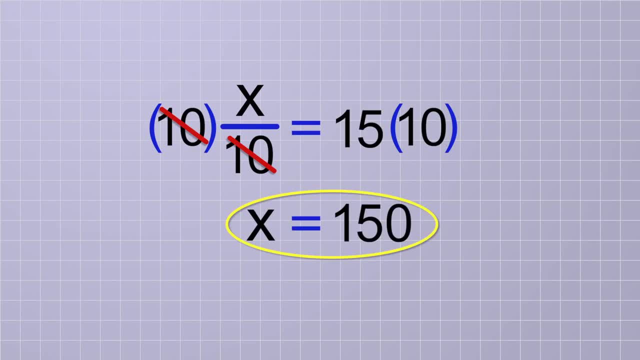 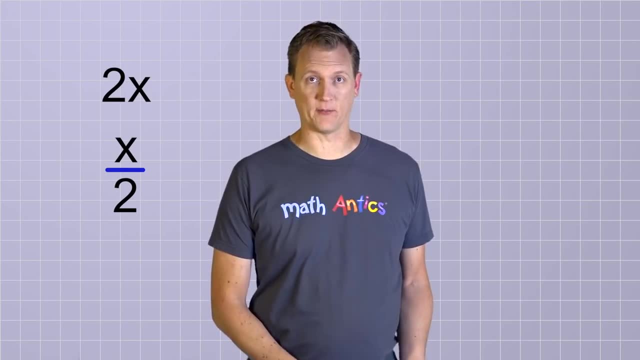 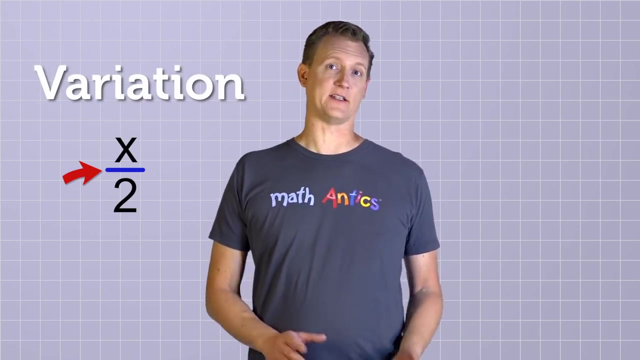 So our answer is: x equals 150.. Great, That's how you solve simple equations where an unknown is being multiplied by a number or divided by a number. But, just like with subtraction in the last video, with division there's a tricky variation that I need to tell you about. 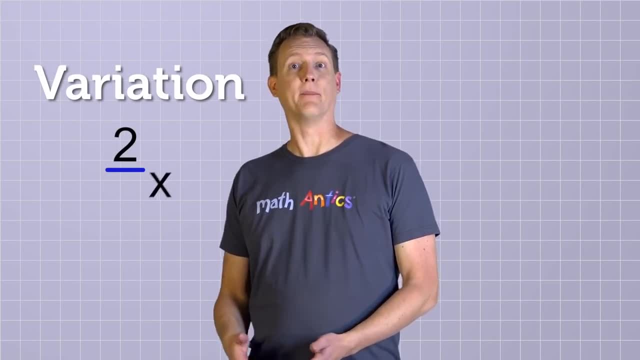 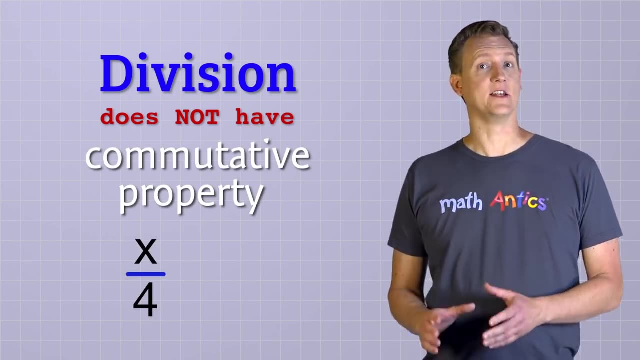 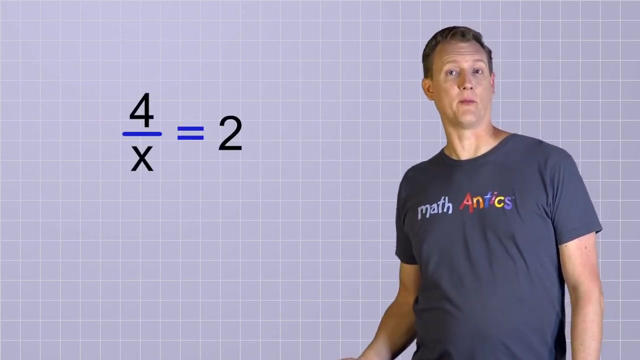 What if you have an equation where a number is being multiplied by a number Or is being divided by an unknown, Since division does not have the commutative property? x over 4 is NOT the same thing as 4 over x. So what do we do if the unknown is on the bottom, like in this problem? 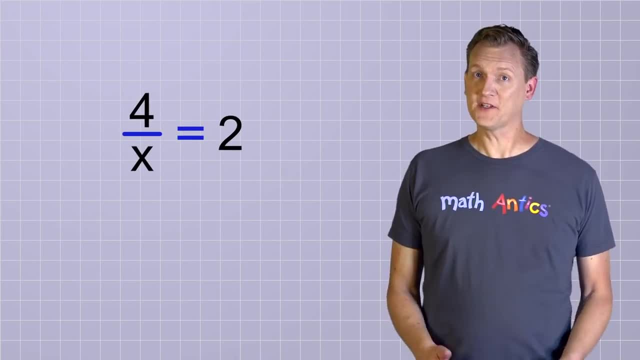 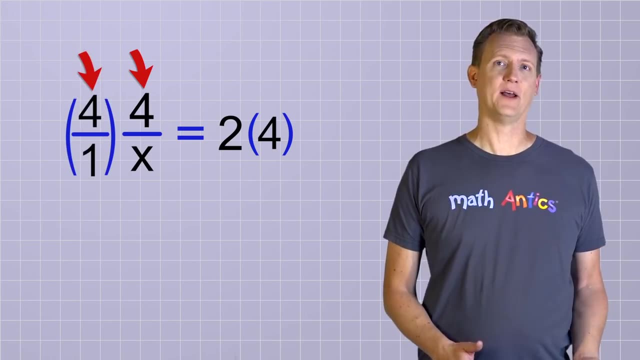 4 over x equals 2.. Well, your first thought might be to multiply both sides by 4.. But that won't help us here, because both of the 4's would be on top, so they wouldn't cancel each other out. 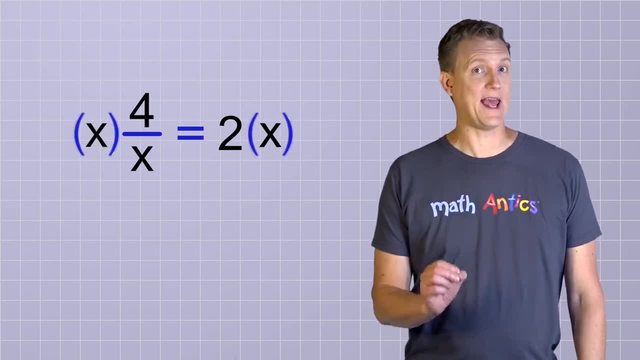 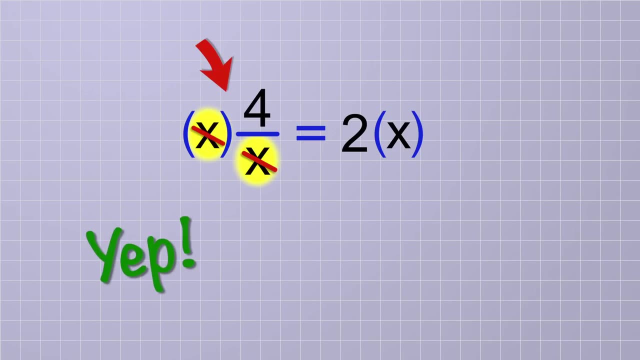 Instead, what we need to do is multiply both sides by x. Watch what happens. then The x's on this side of the equation will cancel. Yep, you can cancel unknowns and variables exactly like you can regular numbers. That will leave us with just 4 on this side of the equation. 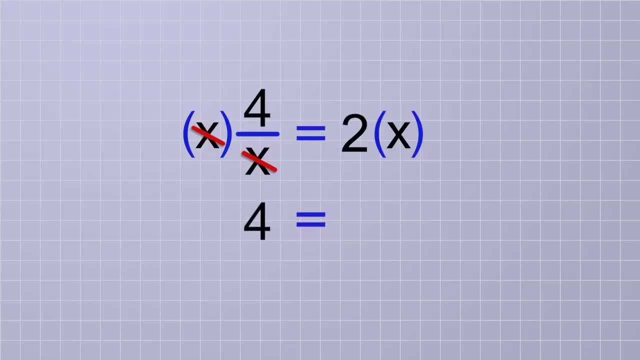 And on the other side we have 2 times x or 2x. True, that didn't solve the equation, but it did get rid of the tricky x on the bottom. True, that didn't solve the equation, but it did get rid of the tricky x on the bottom.